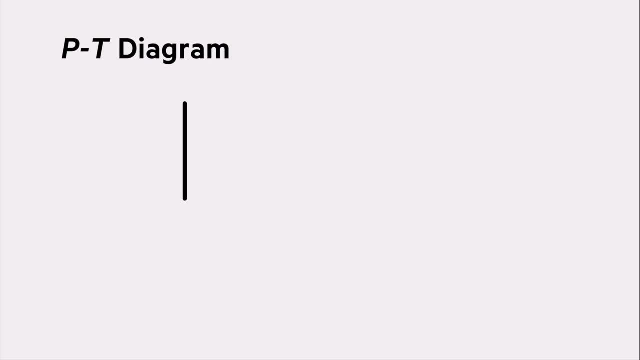 diagram called the P-T diagram. This graph shows the location of the different phases of a pure substance in relation to pressure and temperature, with pressure P on the vertical axis and the temperature T on the horizontal axis. The three phases are separated from each other by so-called separation lines. 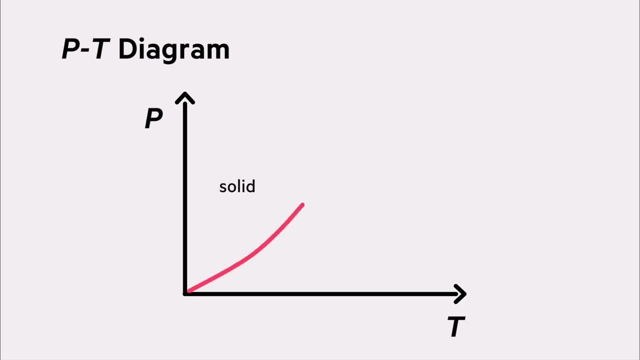 We have the sublimation line which divides the solid and the vapor phase. The sublimation line ends at the triple point, which is the point where all three phases coexist. There is a melting line between the solid and the liquid phase and the vaporization. 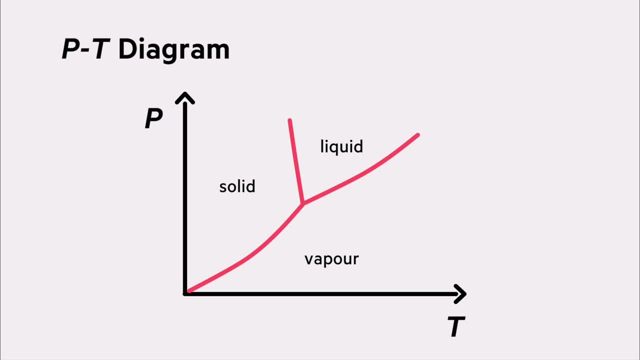 line between the liquid and the gaseous phase. The vaporization line ends in the critical point. Sublimation occurs when a substance crosses the sublimation line from here to here. The other way around, the desublimation, or deposition, happens when the substance goes. 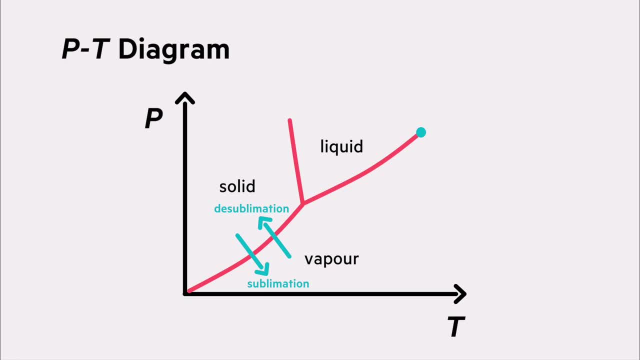 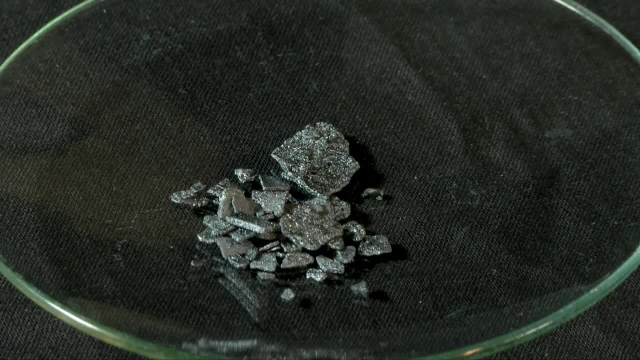 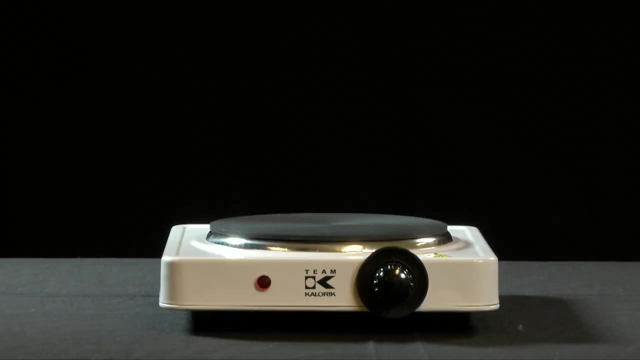 from the vapor phase directly into the solid phase. Let's turn from theory to practice. We are going to turn solid iodine directly into gas and then reverse it back from gas to solid, without the iodine ever being in a liquid state. We will use a heating plate, a beaker, a watch glass, ice cubes and some solid iodine. 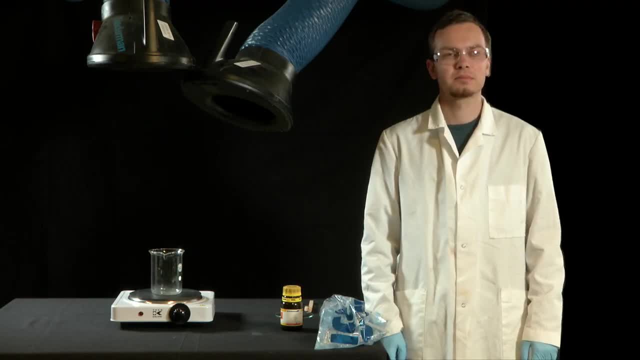 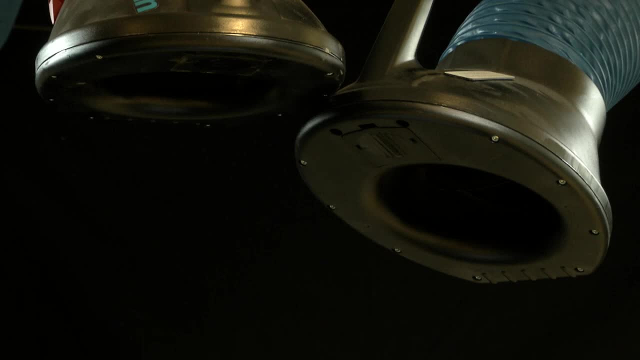 But remember: Iodine, both in solid and gaseous phase, can be toxic. To handle iodine you need both goggles and gloves. You also need a fume hut to ventilate and prevent a high concentration of gaseous iodine. 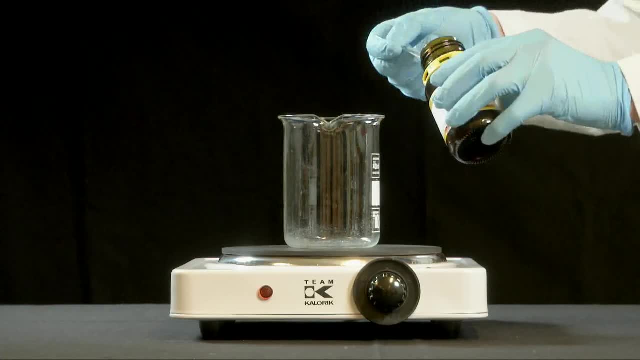 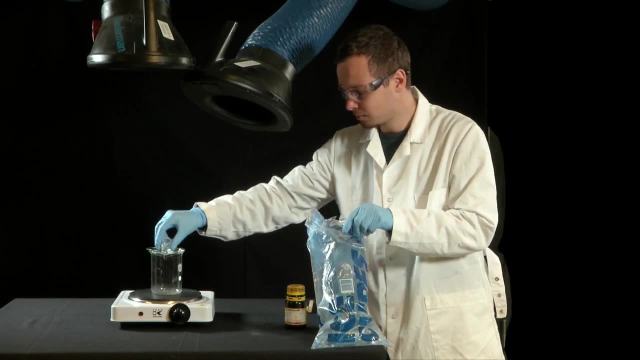 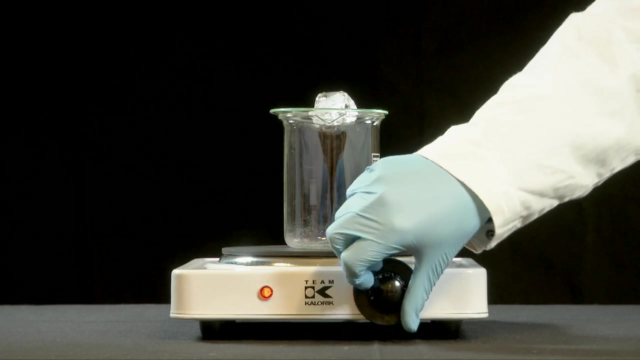 in the room. We put just a few teaspoons of solid iodine into the beaker. The watch glass then goes on top of the beaker and we place some ice cubes onto the watch glass in order to keep it cold. We are ready to start applying heat. 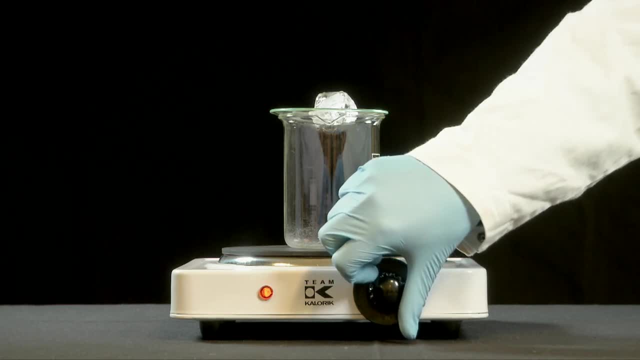 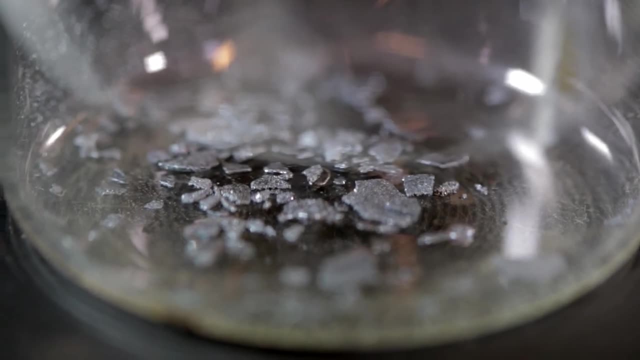 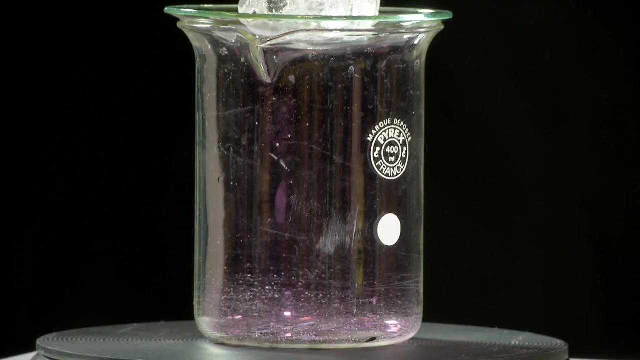 This will accelerate the process. The experiment starts at one atmosphere, which is the general air pressure around us, and at room temperature, which is about 22 degrees Celsius. The temperature rises and the purple gas starts to appear. This means that sublimation is occurring.